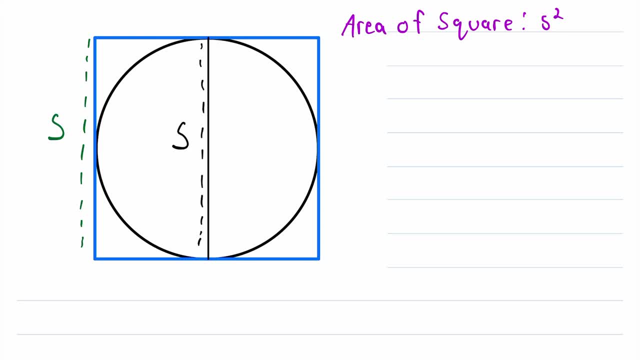 So this diameter length of this circle is S. And if the diameter length is S, what does that tell us about the diameter of the circle? What does that tell us about the radius, this brown segment here? Well, the radius is half of the diameter, so the radius has to be S over 2.. 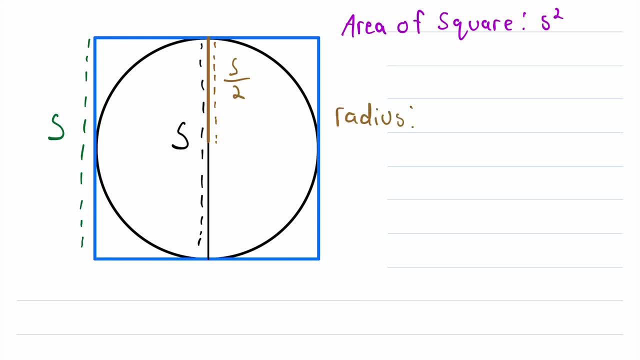 And just in case that diagram is a little hard to read, I'll just write that over here. The radius length of our circle is S over 2. That's half the side length of the square that it is inscribed in. Alright, so that tells us the second area that we might be concerned with. 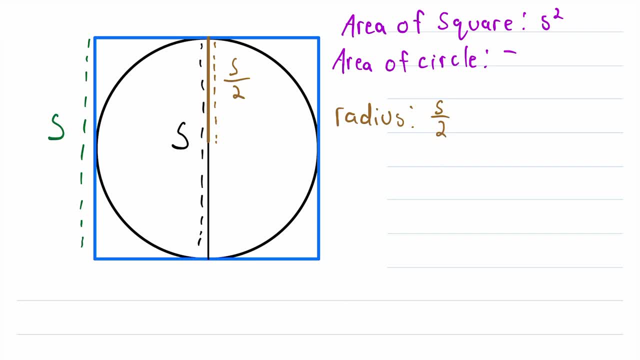 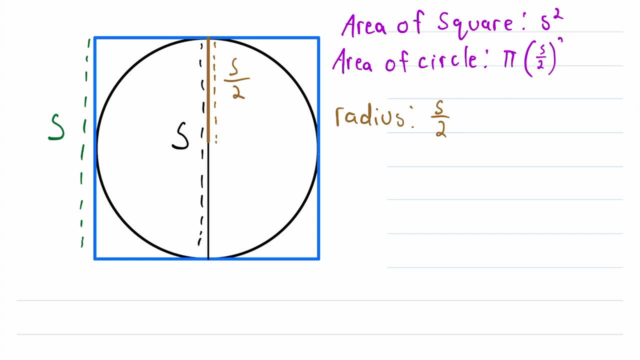 The radius is S over 2, so that's pi S over 2 squared. Alright, now let me just move this writing down a little bit. Then the other area we might be concerned with is this area that I'm shading in green. 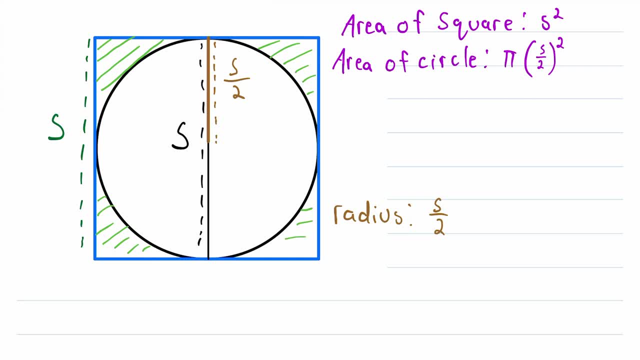 This is the area that's inside the square but outside the circle. So how can we find that area? Well, it's pretty easy. Let me first shade the area of the square. So what I've just shaded is the area of the square which, remember, is S squared. 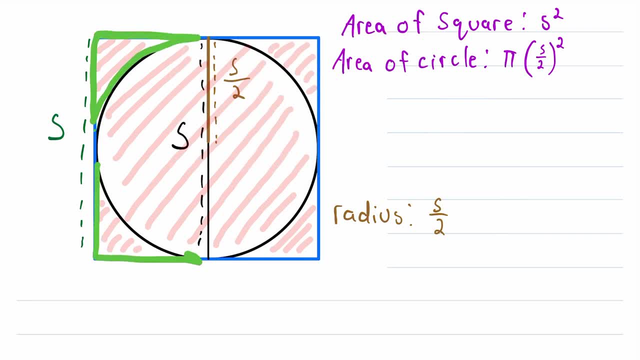 So if we want the area of these sort of triangular sections, you might be able to tell that all we need to do is take the area of the square and then remove the area of the circle. So what I just had shaded was the area of the whole square. 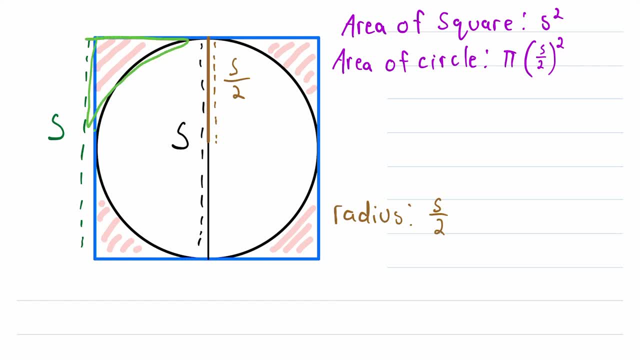 then I removed the area of the circle and you can see that what I have remaining is the area that's inside the square but outside the circle. So let me write that here, To find the area in the square but outside of the circle. 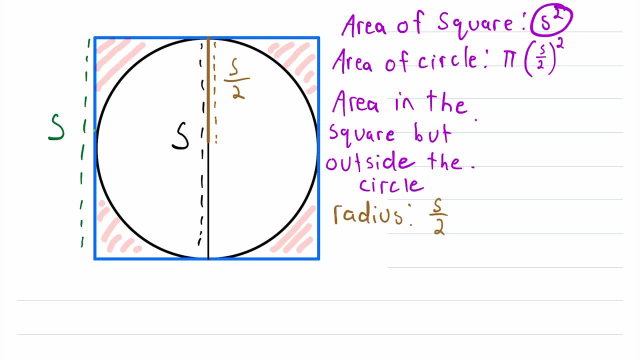 all we need to do to calculate that area is: take the area of the whole square, which is S squared, and then subtract the area of the inscribed circle, which is pi times S over 2 squared. So that's minus pi times S over 2 squared. 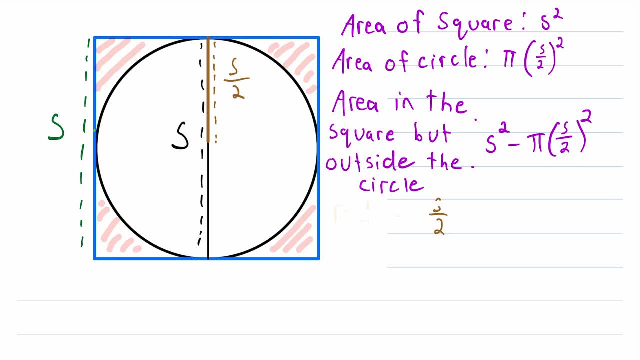 And I'm just going to erase that, Erase this remark about the radius here, so we have a little bit more room, Alright, so that's not all too tricky, is it? We've got a square with side length S. The area of the square is S squared. 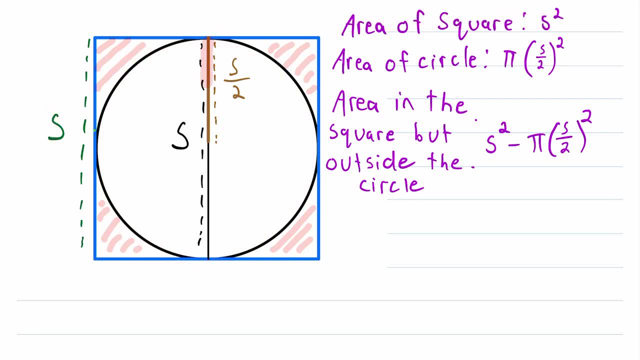 And then we have a circle inscribed in that square. The diameter length of the circle is the side length of the square that it's inscribed in, which is S, which means that the radius has a length of S over 2.. So the area of the circle inscribed in the square 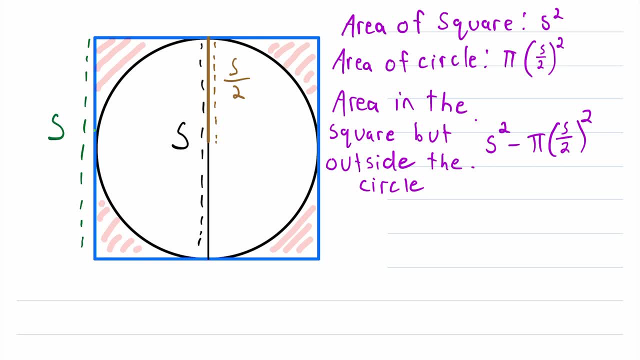 is pi times S over 2 squared. Then to find the area that's in the square but outside the circle, we just have to take the area of the square S squared and subtract the area in the circle, which is pi times S over 2 squared. 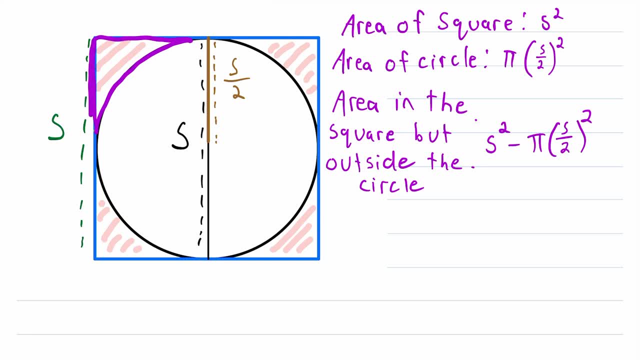 Then also, if you wanted to find the area of just one of these vaguely triangular sections, well, this expression over here gives you the area of all four of those sort of triangular sections, And since they're all congruent, if you only want the area of one of them, 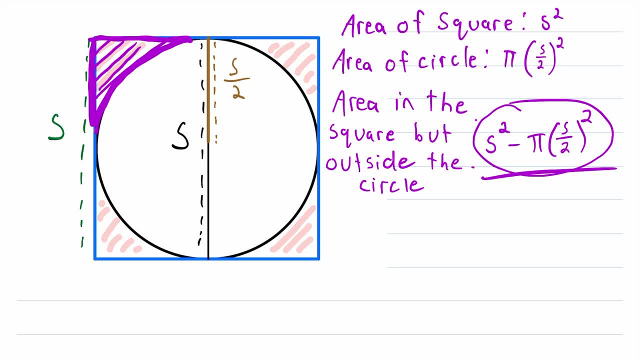 you just have to take this total area expression and divide it by 4.. I'm not going to write that down, but just remember that these four sections are congruent. So if you ever need to find the area of just one of them or just two of them, 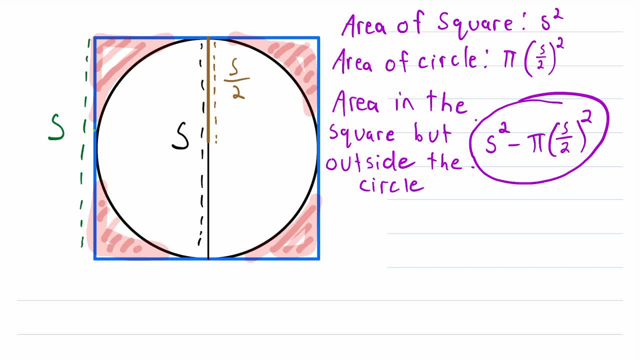 you can just use this expression for the area of all of them, but do the necessary division, Alright. so that's really all there is to it for these area calculations, And I suppose before we go, we'll do an example. So let's say that the side length of this square is, let's say, 8 centimeters. 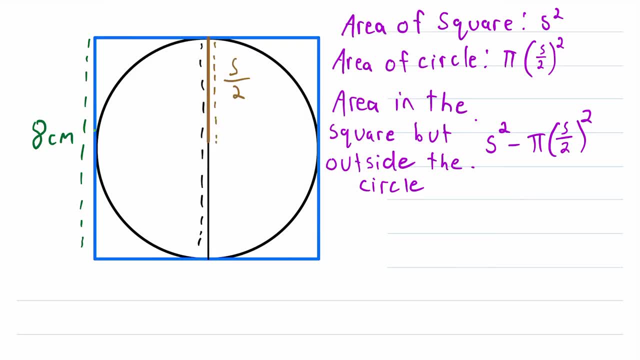 So then, the diameter length of this circle is also 8 centimeters. That means the radius length is 8 centimeters over 2, which is just 4 centimeters. Alright, so then, first, what's the area of the square? 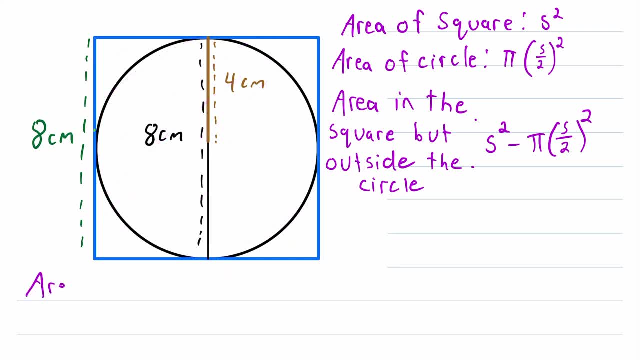 I'll write this down here: The area of the square is equal to the side length squared. The side length is 8 centimeters, so the area of the square is 8 centimeters squared, which is 64 centimeters squared. Then what about the area of the circle?